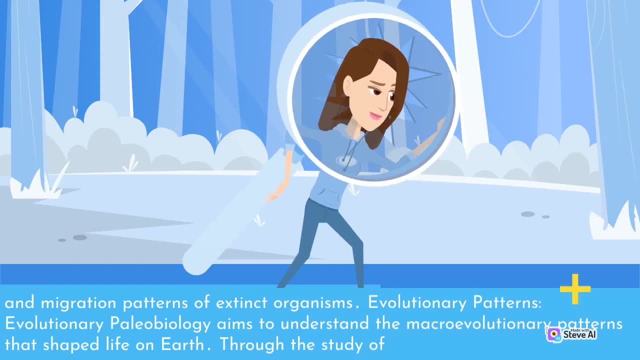 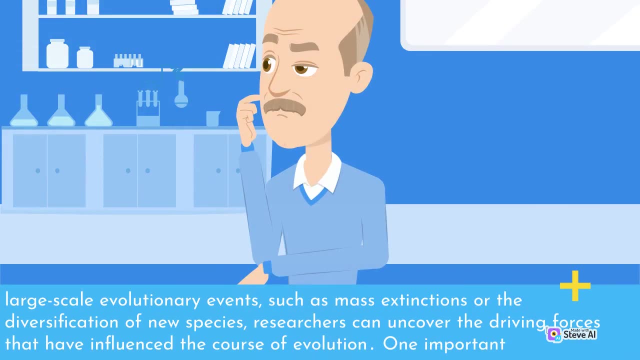 aims to understand the macroevolutionary patterns that shape life on earth. Through the study of large-scale evolutionary events, such as mass extinctions or the diversification of new species, researchers can uncover the driving forces that have influenced the course of evolution. 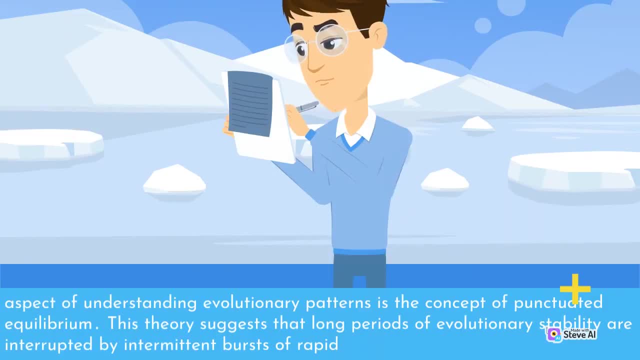 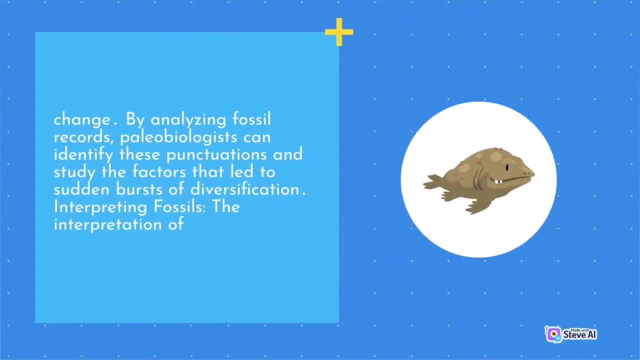 One important aspect of understanding evolutionary patterns is the concept of punctuated equilibrium. This theory suggests that long periods of evolutionary stability are interrupted by intermittent bursts of rapid change. By analyzing fossil records, paleobiologists can identify these punctuations and study the factors that led to sudden bursts of diversification. 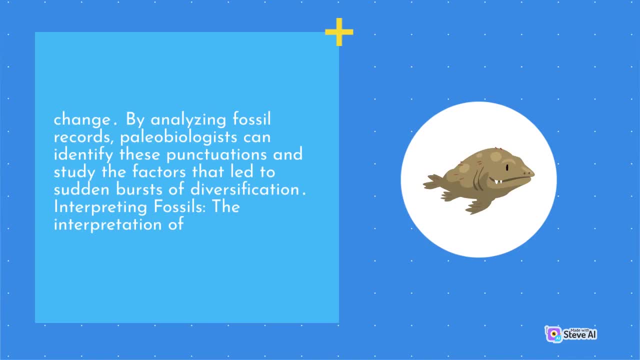 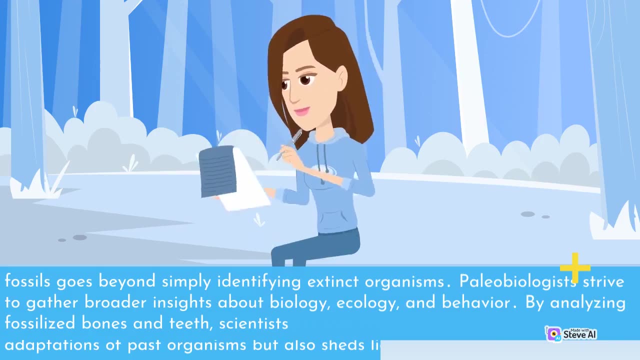 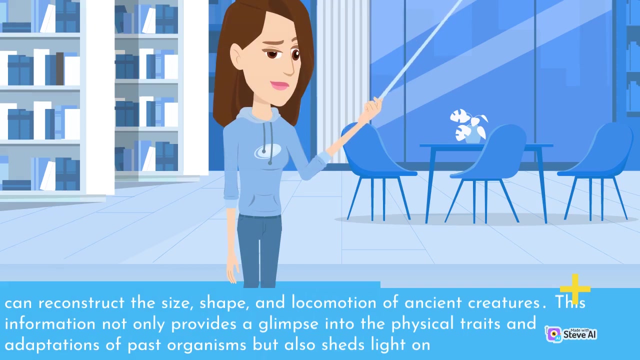 Interpreting fossils. the interpretation of Fossils goes beyond simply identifying extinct organisms. Paleobiologists strive to gather broader insights about biology, ecology and behavior. By analyzing fossilized bones and teeth, scientists can reconstruct the size, shape and locomotion of ancient creatures. 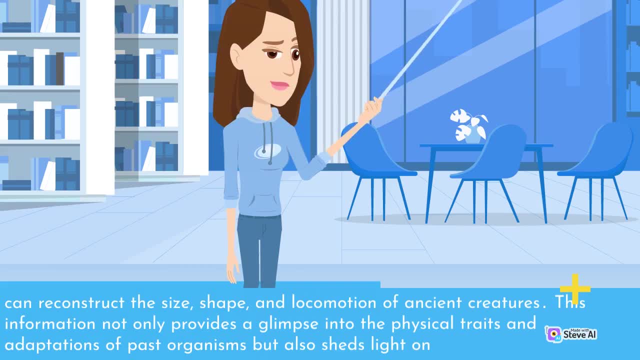 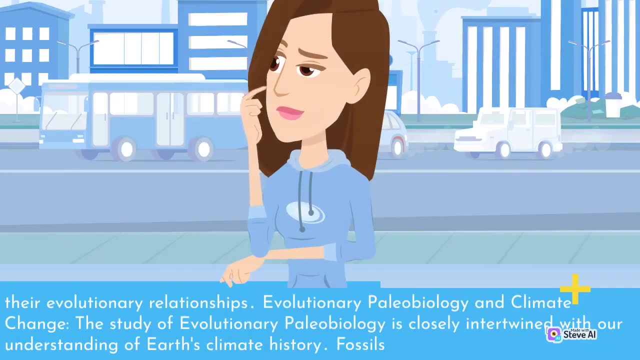 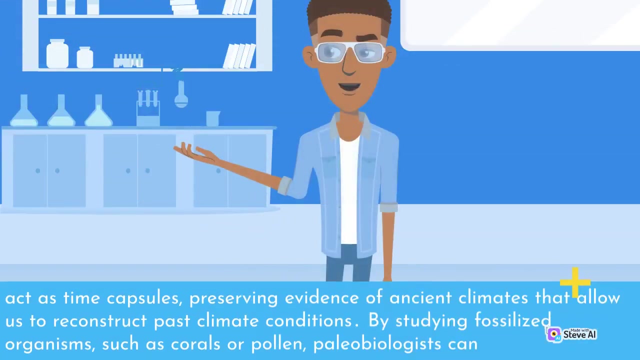 This information not only provides a glimpse into the physical traits and adaptations of past organisms, but also the history of the species. The study of fossilized bones and teeth can be hold firm to the civilized balance. In parallel evolution will thus reassemble the most. more complex cancelation systems. This is also a really broad point of Christianity, contemplating the acceptance of certain underground actions, such as the power of skydiving, the dispatch and calm of migration and global science of possible means of發 azooma or Me uniforms and might createfound world bipolar. 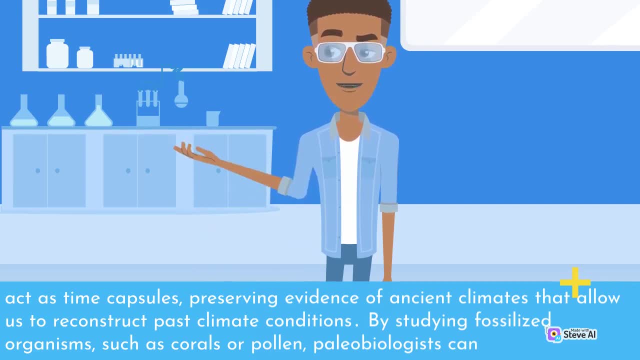 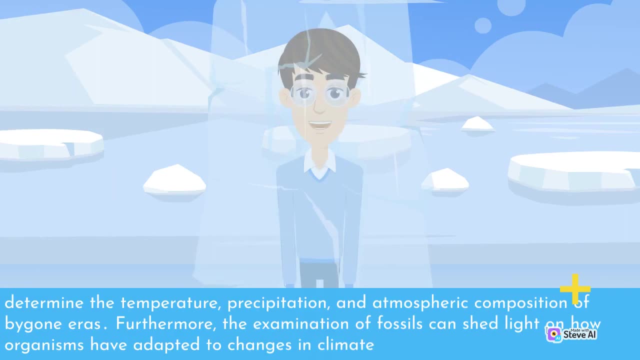 dynamics such that these together can turn orbital events into series of events understood along cultural, economic basis for the audience. incident has also shed light on paleobiologists can determine the temperature, precipitation and atmospheric composition of bygone eras. Furthermore, the examination of fossils can shed light on how organisms have 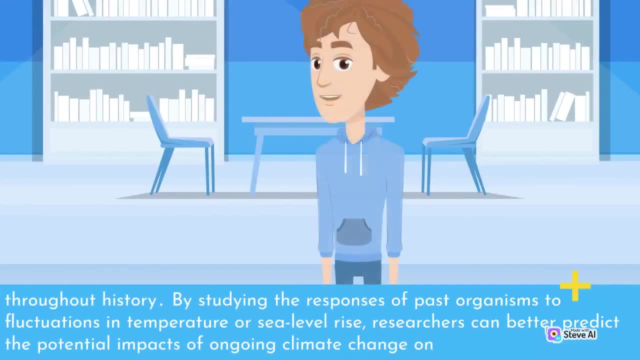 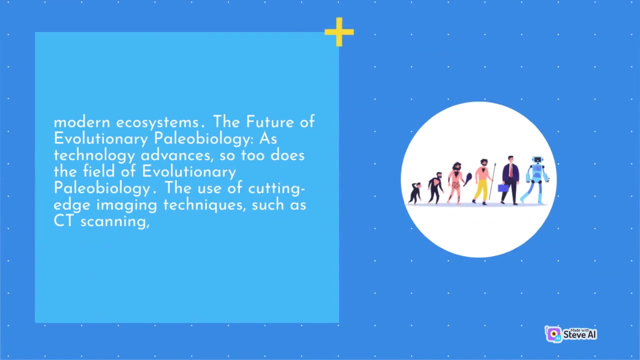 adapted to changes in climate throughout history. By studying the responses of past organisms to fluctuations in temperature or sea level rise, researchers can better predict the potential impacts of ongoing climate change on modern ecosystems. The future of evolutionary paleobiology. as technology advances, so too does the field of evolutionary paleobiology. 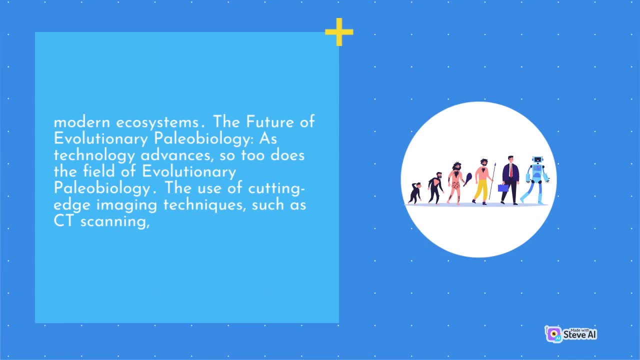 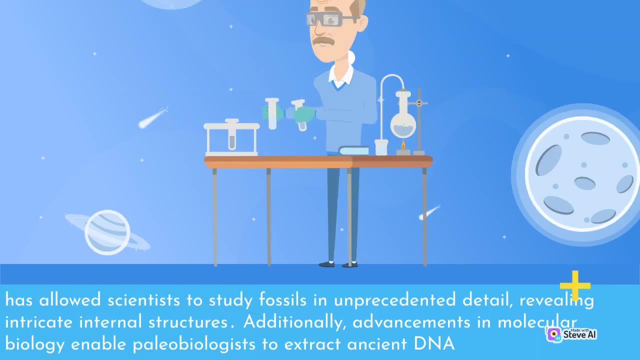 The use of cutting-edge imaging techniques such as CT scanning has allowed scientists to study fossils in unprecedented detail, revealing intricate internal structures. Additionally, advancements in molecular biology have been made possible by the use of cutting-edge imaging techniques such as CT scanning. 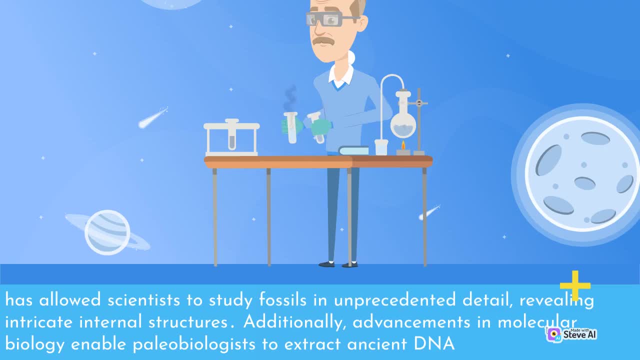 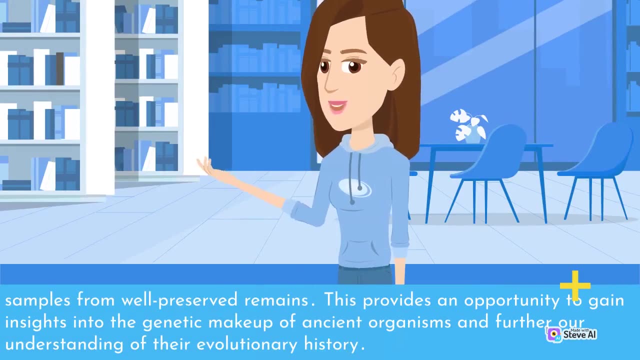 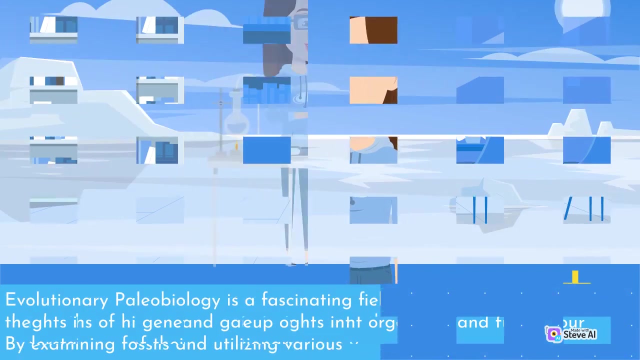 The use of cutting-edge imaging techniques such as CT scanning enables paleobiologists to extract ancient DNA samples from well-preserved remains. This provides an opportunity to gain insights into the genetic makeup of ancient organisms and further our understanding of their evolutionary history. Evolutionary paleobiology is a fascinating field that 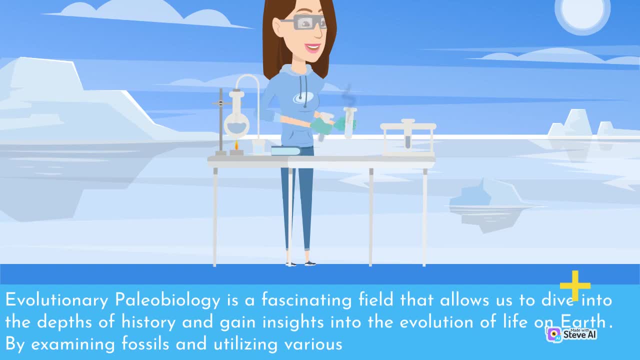 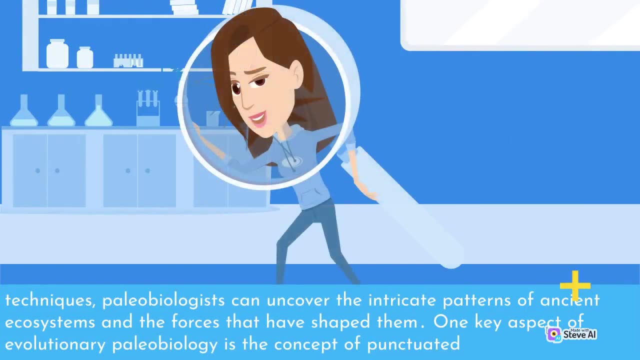 allows us to dive into the depths of history and gain insights into the evolution of life on Earth. by examining fossils and utilizing various techniques, Paleobiologists can uncover the intricate patterns of ancient ecosystems and the forces that have shaped them. One key aspect of evolutionary paleobiology is the concept of 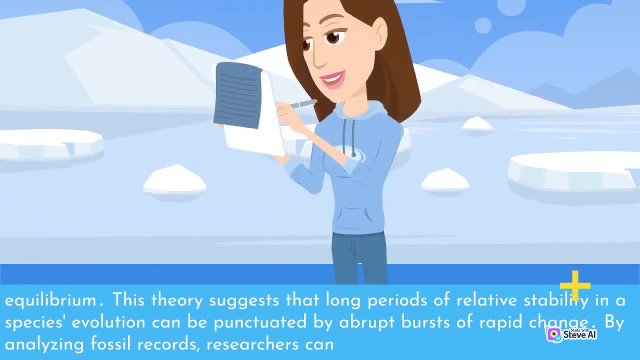 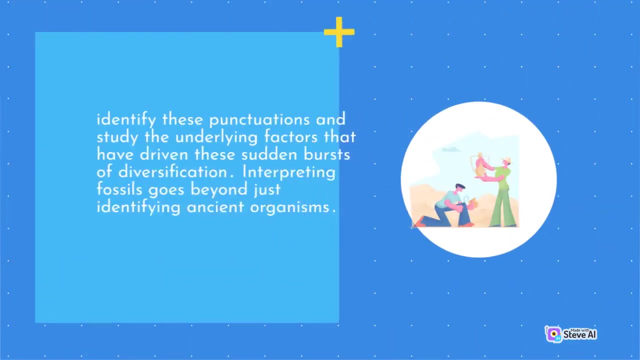 punctuated Equilibrium. This theory suggests that long periods of relative stability in a species evolution can be punctuated by abrupt bursts of rapid change. By analyzing fossil records, researchers can identify these punctuations and study the underlying factors that have driven these. 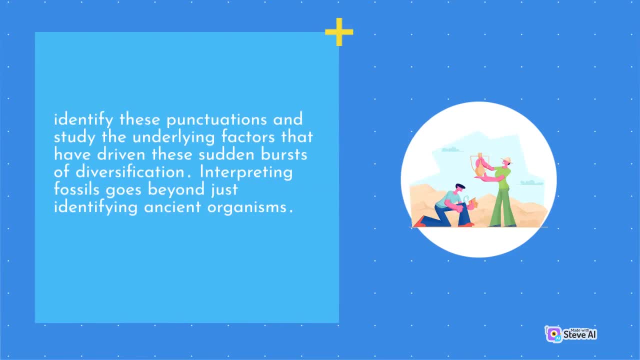 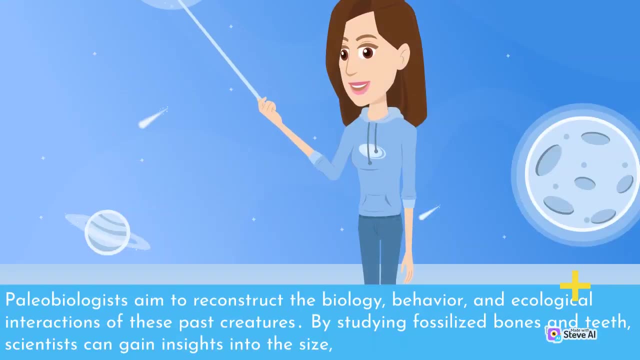 sudden bursts of diversification. Interpreting fossils goes beyond just identifying ancient organisms. Paleobiologists aim to reconstruct the biology, behavior and ecological interactions of these past creatures. By studying fossilized bones and teeth, scientists can gain insights into the size 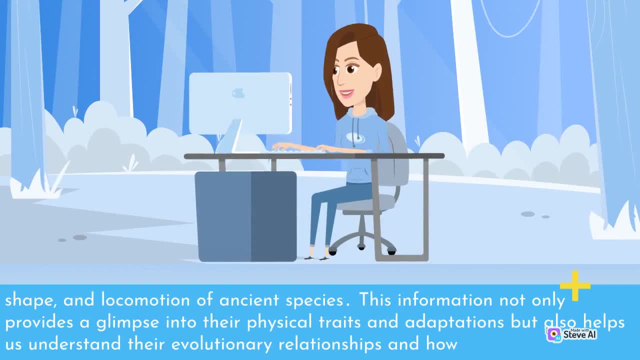 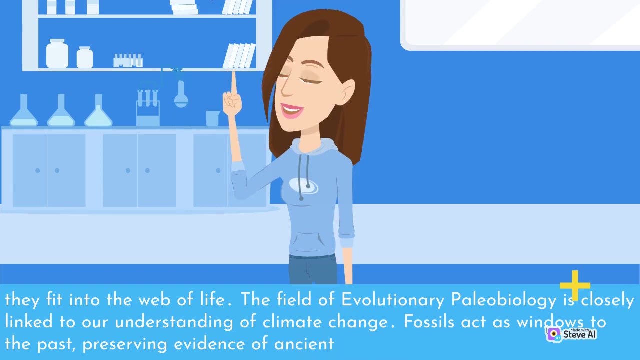 shape and length of the species and locomotion of ancient species. This information not only provides a glimpse into their physical traits and adaptations, but also helps us understand their evolutionary relationships and how They fit into the web of life. The field of evolutionary paleobiology is closely linked to 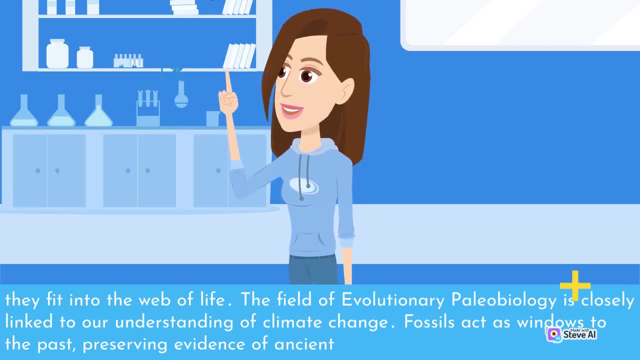 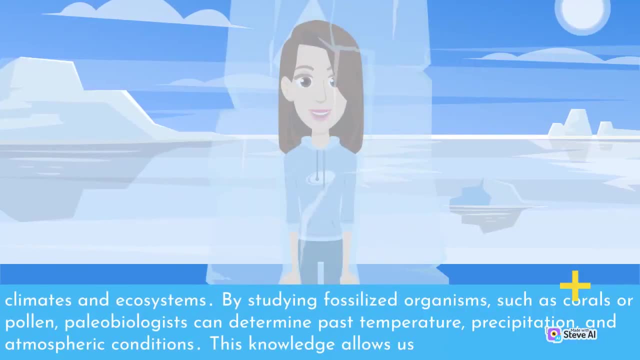 our understanding of climate change. Fossils act as windows to the past, preserving evidence of ancient Climates and Ecosystems. By studying fossilized organisms such as corals or pollen, paleobiologists can determine past temperature, precipitation and atmospheric conditions. 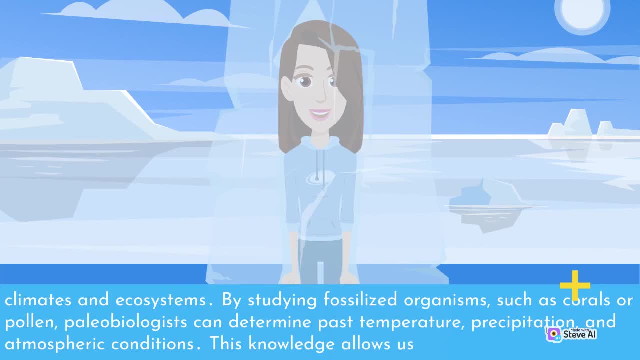 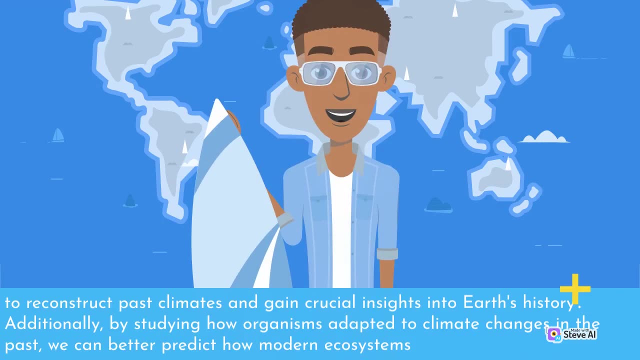 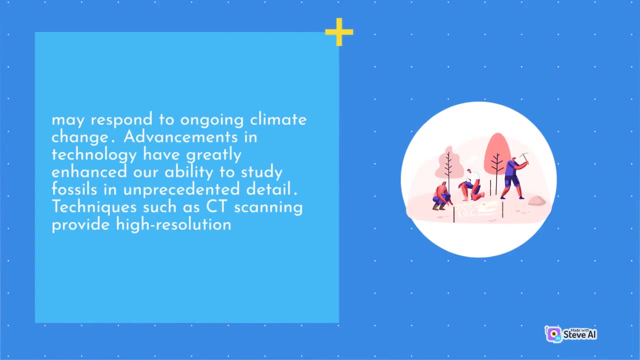 This knowledge allows us to reconstruct past climates and gain crucial insights into Earth's history. Additionally, by studying how organisms adapted to climate changes in the past, we can better predict how modern ecosystems may respond to ongoing climate change. Advancements in technology have greatly enhanced our ability to study fossils in unprecedented detail. 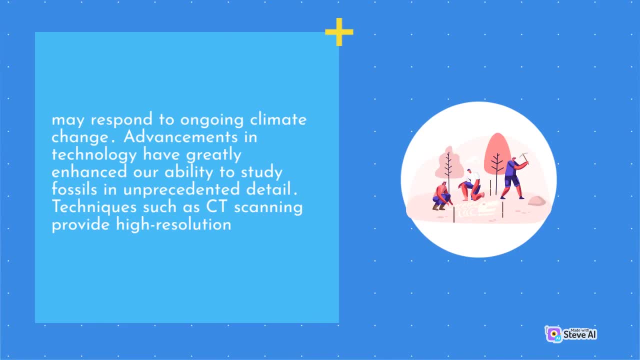 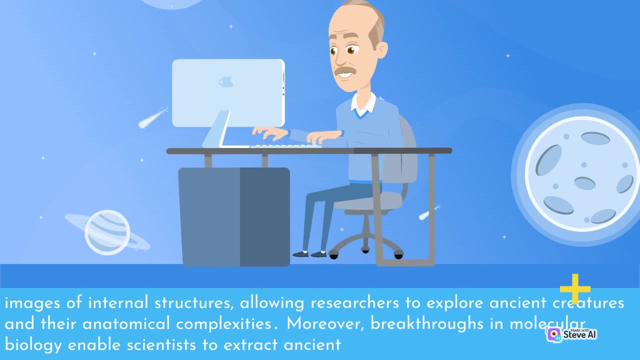 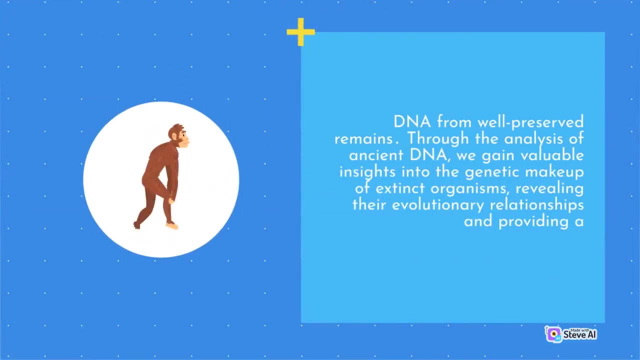 Techniques such as CT scanning provide high resolution Images of internal structures, allowing researchers to explore ancient creatures and their anatomical complexities. Moreover, breakthroughs in molecular biology enable scientists to extract ancient DNA from well-preserved fossils- DNA from well-preserved remains. Through the analysis of ancient DNA, we gain valuable insights into the genetic makeup of extinct organisms, revealing their evolutionary relationships and providing a 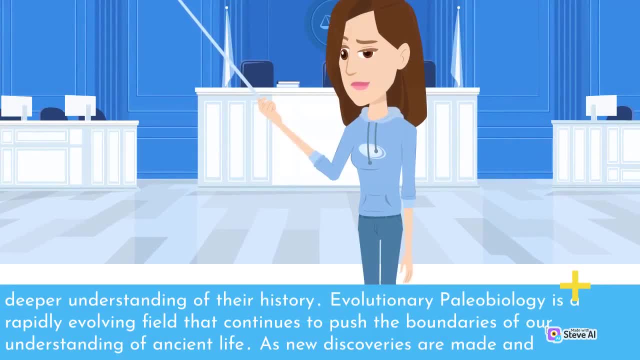 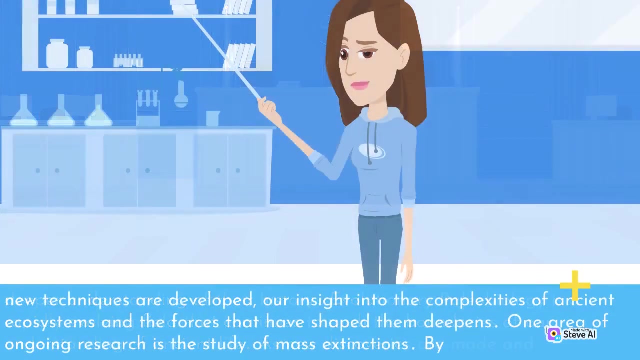 deeper understanding of their history. Evolutionary paleobiology is a rapidly evolving field that continues to push the boundaries of our understanding of ancient life As new discoveries are made and new technologies are created. New techniques are developed. our insight into the complexities of ancient ecosystems and the forces that have shaped them deepens. One area of ongoing research is the study of mass extinctions. 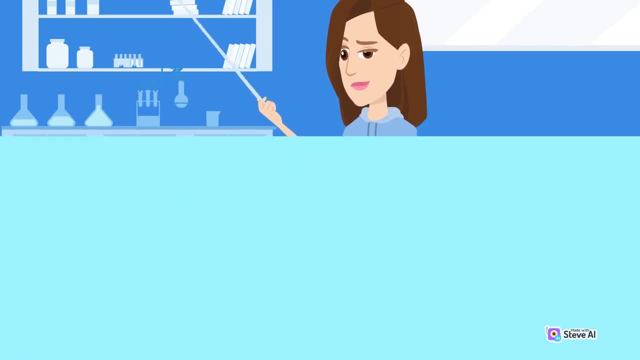 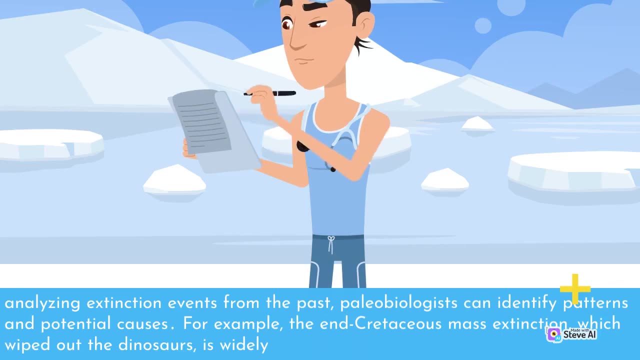 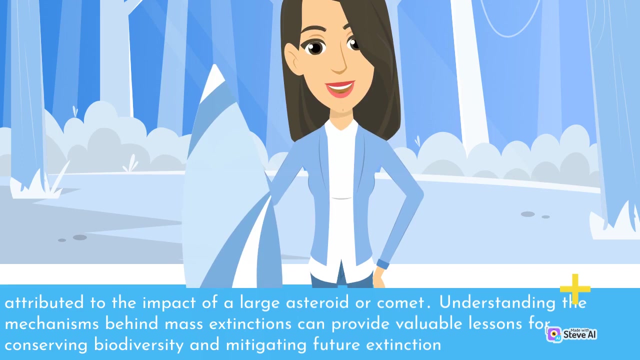 By Analyzing extinction events from the past, paleobiologists can identify patterns and potential causes. For example, the end Cretaceous mass extinction, which wiped out the dinosaurs, is widely analyzed Attributed to the impact of a large asteroid or comet. Understanding the mechanisms behind mass extinctions can provide valuable lessons for conserving biodiversity and mitigating future extinction. 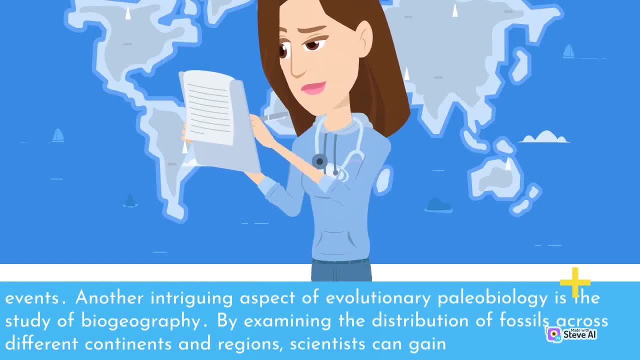 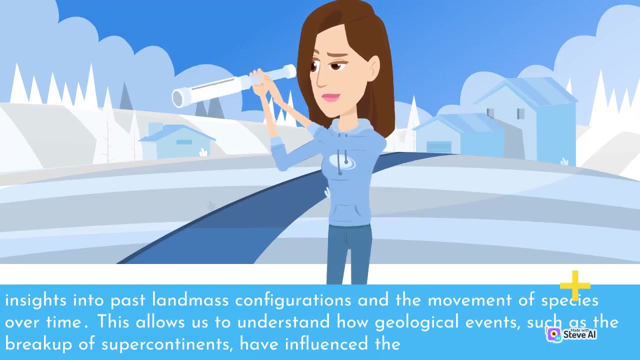 Events. Another intriguing aspect of evolutionary paleobiology is the study of biogeography. By examining the distribution of fossils across different continents and regions, scientists can gain insights into past land mass configurations and the movement of species over time. This allows us to understand how geological events such as the breakup of supercontinents have influenced the 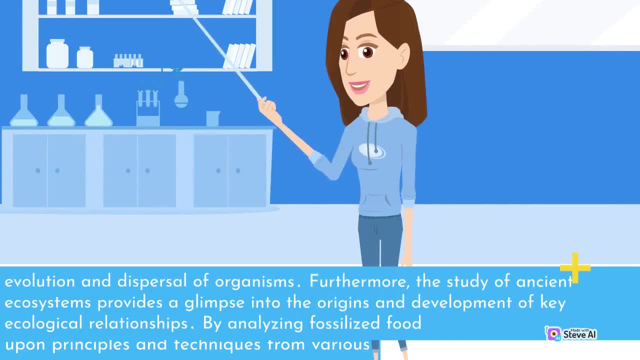 evolution and dispersal of organisms. Furthermore, the study of ancient ecosystems provides a glimpse into the origins and development of key ecological relationships By analyzing fossilized food, species of different species, of different species of different types. We then unable to understand the history of the world. 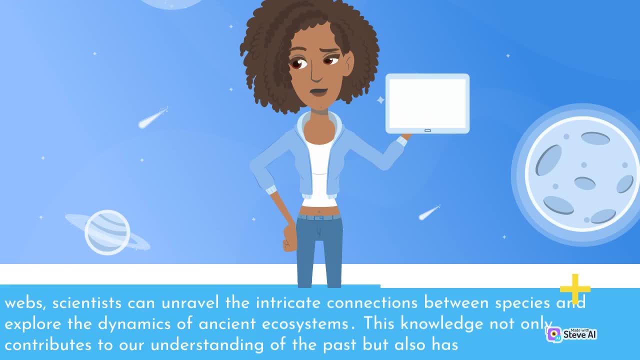 And so we consume an adaptation of ancient ecosystems, And it's possible that the participants who are interested in studying this paradigm can also purchase this material and start studying this field. Scientists can unravel the intricate connections between species and explore the dynamics of ancient ecosystems. This knowledge not only contributes to our understanding of the past, but also has. 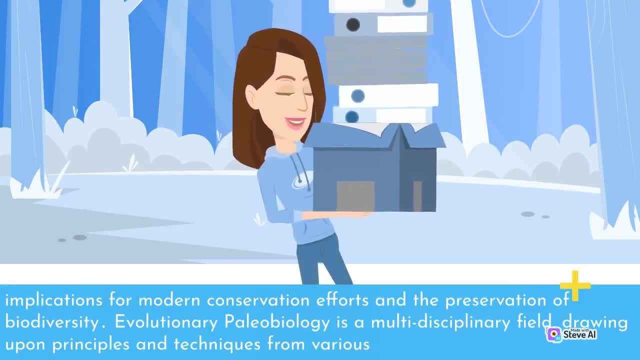 implications for modern conservation efforts and the preservation of biodiversity. Evolutionary paleobiology is a multidisally field, drawing upon principles and techniques from various scientific disciplines. From the beginning, about three hundred thousand lived in a world that had various groups of species, including the species of the animals which contained the most quite. 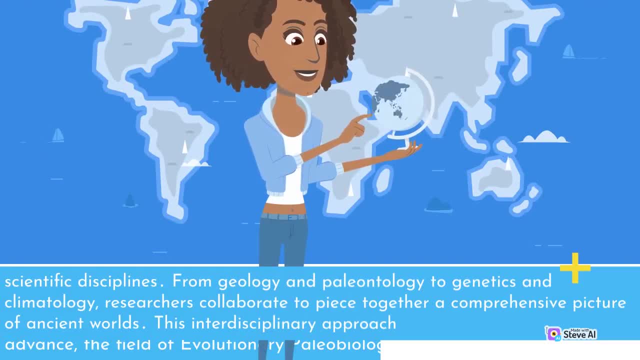 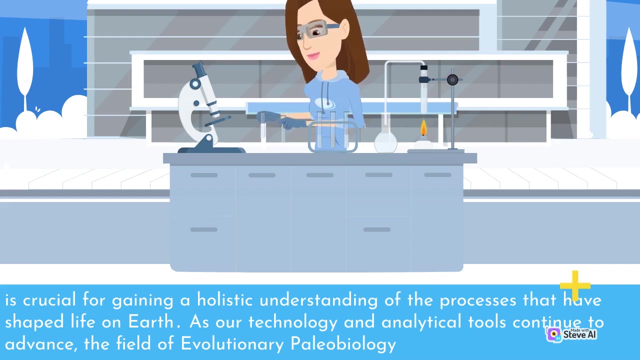 From geology and paleontology to genetics and climatology, researchers collaborate to piece together a comprehensive picture of ancient worlds. This interdisciplinary approach is crucial for gaining a holistic understanding of the processes that have shaped life on Earth. As our technology and analytical tools continue to advance, the field of evolutionary paleobiology. 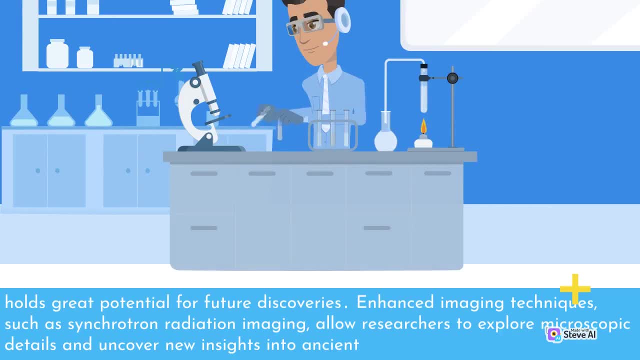 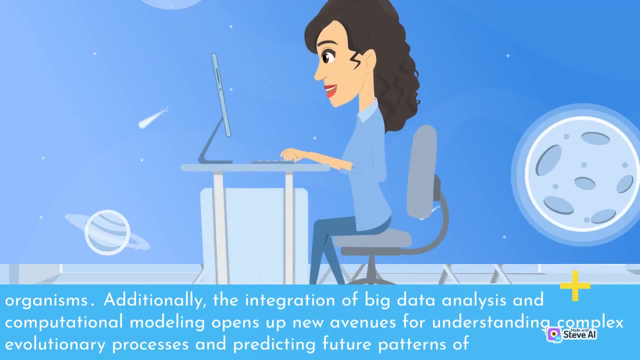 holds great potential for future discoveries. Enhanced imaging techniques, such as synchrotron radiation imaging, allow researchers to explore microscopic details and uncover new insights into ancient organisms. Additionally, the integration of big data analysis and computational modeling opens up new avenues for understanding complex evolutionary processes and predicting future patterns of 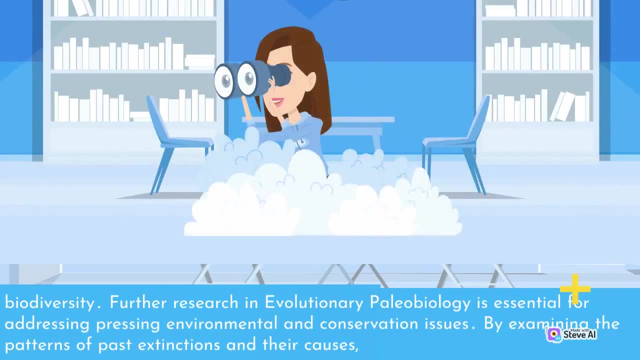 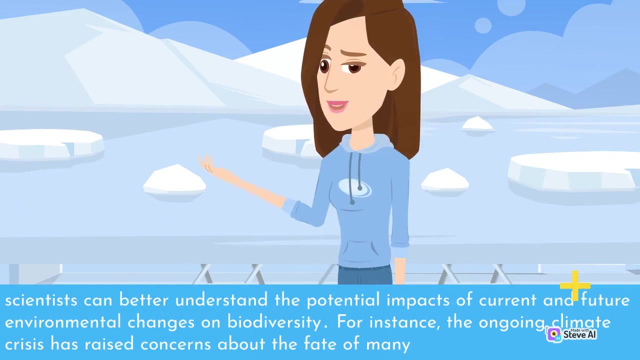 evolution Biodiversity. Further research in evolutionary paleobiology is essential for addressing pressing environmental and conservation issues. By examining the patterns of past extinctions and their causes, scientists can better understand the potential impacts of current and future environmental changes on biodiversity. For instance, the ongoing climate crisis has raised concerns about the fate of many